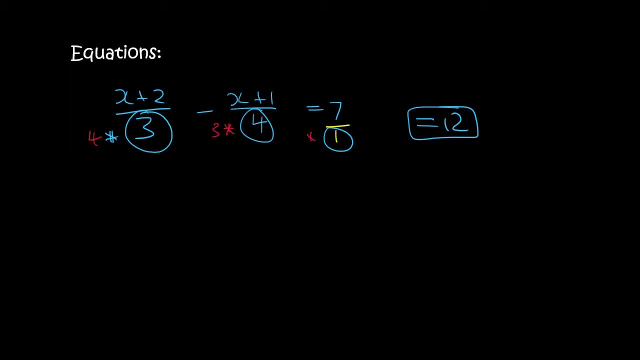 This one is going to be multiplied by 3, and this one will have to be multiplied by 12.. So the way that that would look is: this whole term is going to be multiplied by 4, so you can just go 4, bracket x plus 2.. 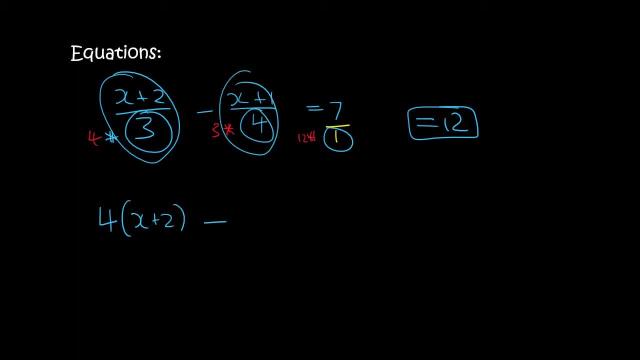 Then you can say minus, then this whole term is being multiplied by 3, so you can say 3, bracket x plus 1, equals to 7.. Or you can say 12,, bracket 7.. You don't need to write the denominators. 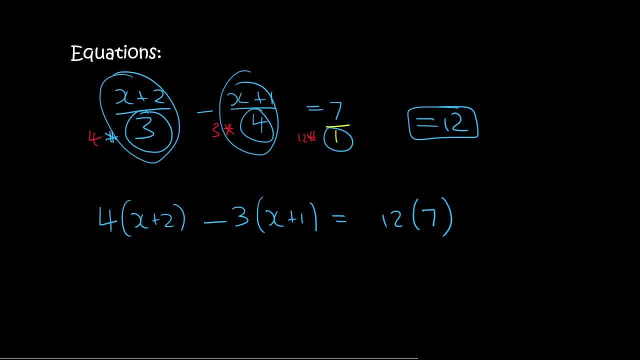 Because it's an equation. And then from this point you just solve like normally. So you multiply the 4 into the brackets. so 4x plus 8, minus 3x minus 3, equals to 84. Then you take all the x's to the one side and all the numbers to the other side. 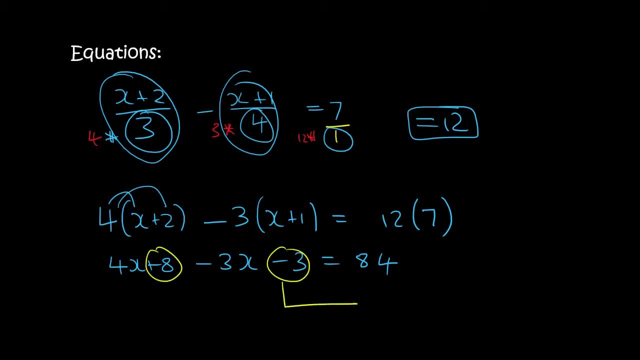 So these two numbers here are going to be moved over to the right, So on the left we'll still have 4x, which is this one, Minus 3x, which is this one, equals 84, which is already there. 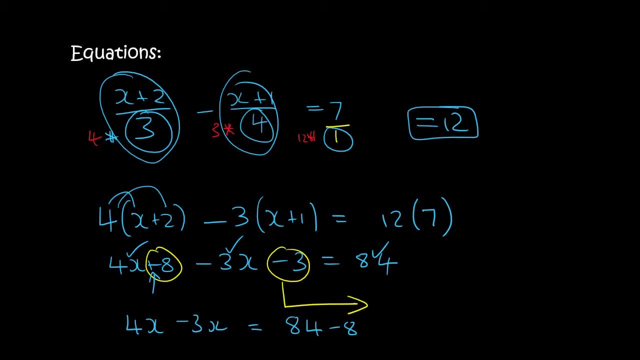 Then this is a plus 8, so it's going to turn to a minus 8.. And this is a minus 3, so it's going to end up being a plus 3.. Then 4x minus 3x is just 1x. 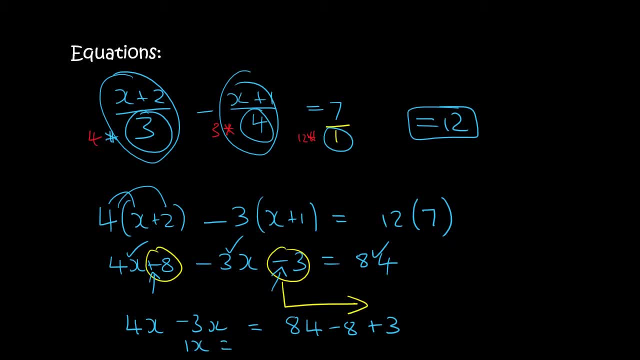 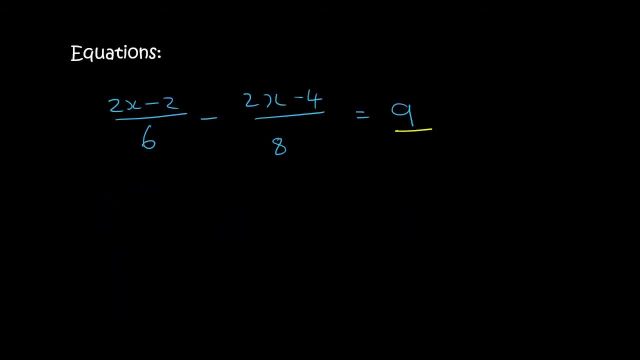 And then 84 minus 8 plus 3, you could do that all in the calculator and that would be 79. So here's another one. So always remember that this 9 is actually 9 over 1.. Now if you look at the numbers 6,, 8, and 1,, a common denominator would be 24.. 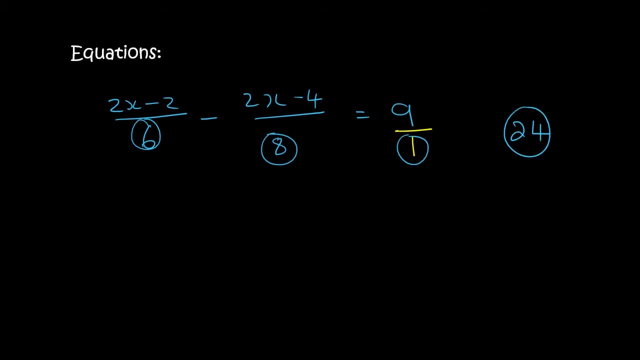 Let's say you missed 24.. Let's say you said 48.. That's absolutely okay, You will still get the same answer. So don't let anyone tell you that it always has to be the lowest one. It can be higher. 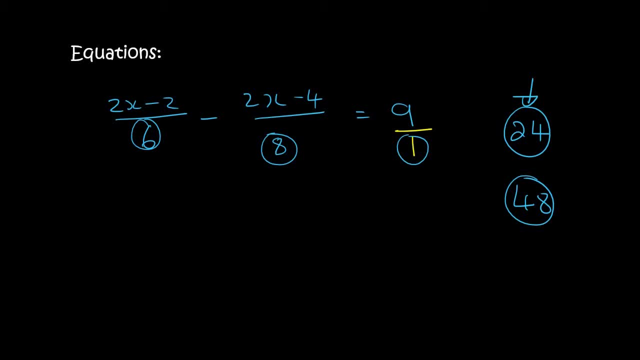 All that happens is the numbers you're going to be working with will be a little bit bigger, But then at the end you will simplify, You'll answer and you'll get the same answer. Okay, so to get to 24, we're going to have to multiply this one by 4, because 6 times 4 is 24.. 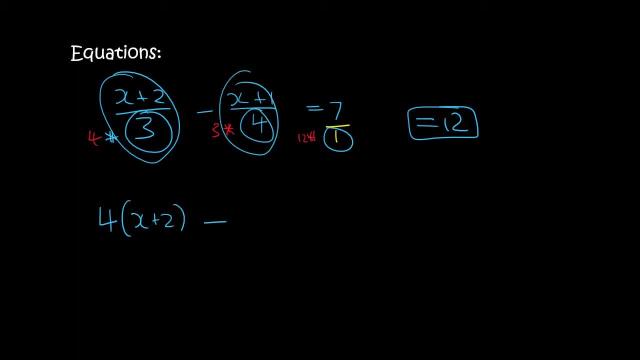 Then you can say minus, then this whole term is being multiplied by 3, so you can say 3, bracket x plus 1, equals to 7.. Or you can say 12,, bracket 7.. You don't need to write the denominators. 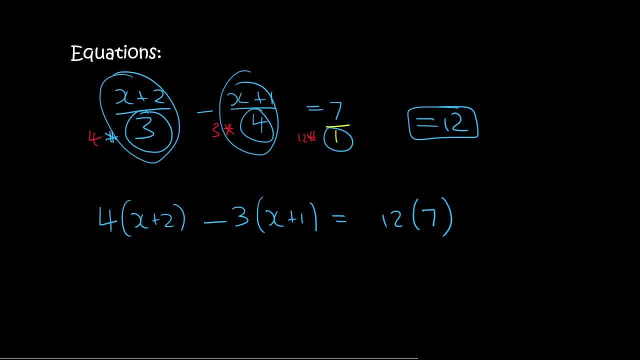 Because it's an equation. And then from this point you just solve like normally. So you multiply the 4 into the brackets. so 4x plus 8, minus 3x minus 3, equals to 84. Then you take all the x's to the one side and all the numbers to the other side. 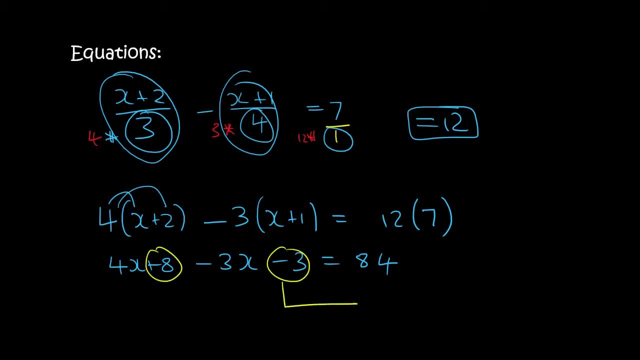 So these two numbers here are going to be moved over to the right, So on the left we'll still have 4x, which is this one, Minus 3x, which is this one, equals 84, which is already there. 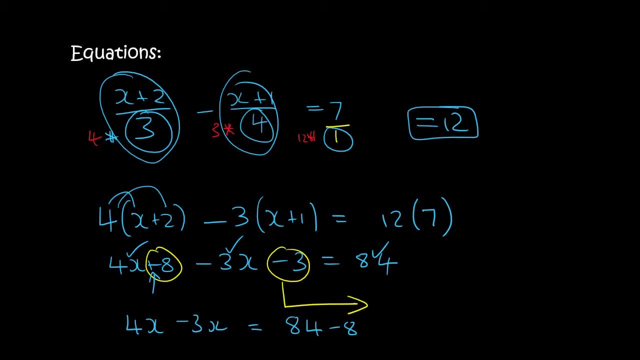 Then this is a plus 8, so it's going to turn to a minus 8.. And this is a minus 3, so it's going to end up being a plus 3.. Then 4x minus 3x is just 1x. 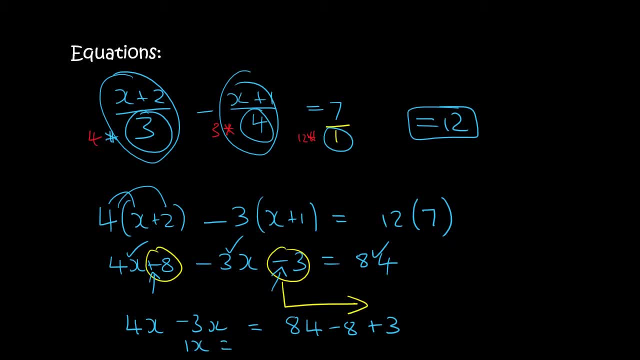 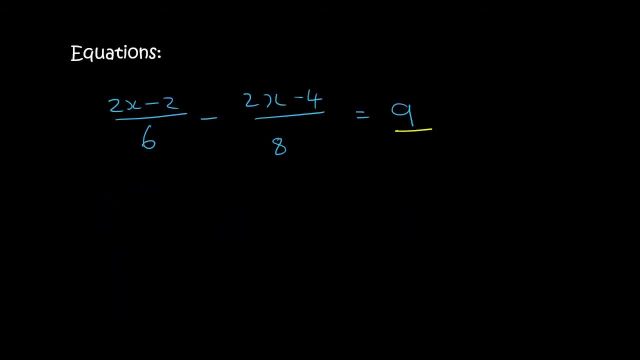 And then 84 minus 8 plus 3, you could do that all in the calculator and that would be 79. So here's another one. So always remember that this 9 is actually 9 over 1.. Now if you look at the numbers 6,, 8, and 1,, a common denominator would be 24.. 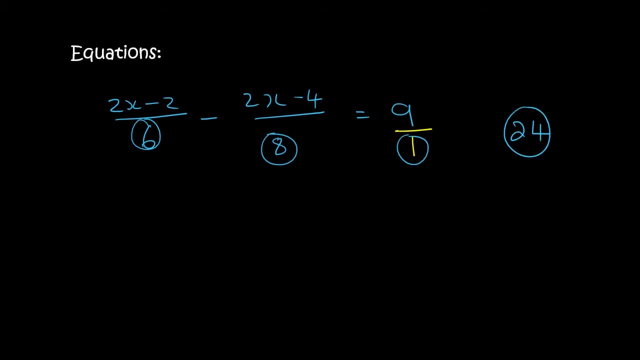 Let's say you missed 24.. Let's say you said 48.. That's absolutely okay, You will still get the same answer. So don't let anyone tell you that it always has to be the lowest one. It can be higher. 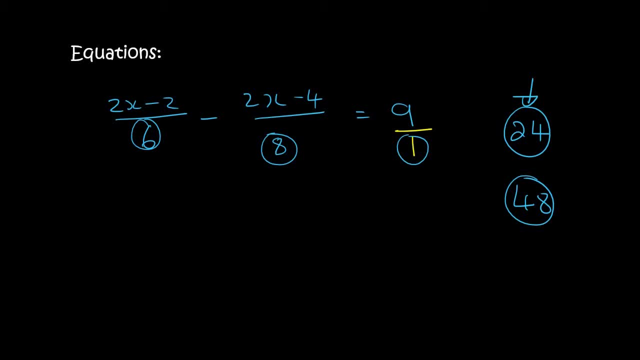 All that happens is the numbers you're going to be working with will be a little bit bigger, But then at the end you will simplify, You'll answer and you'll get the same answer. Okay, so to get to 24, we're going to have to multiply this one by 4, because 6 times 4 is 24.. 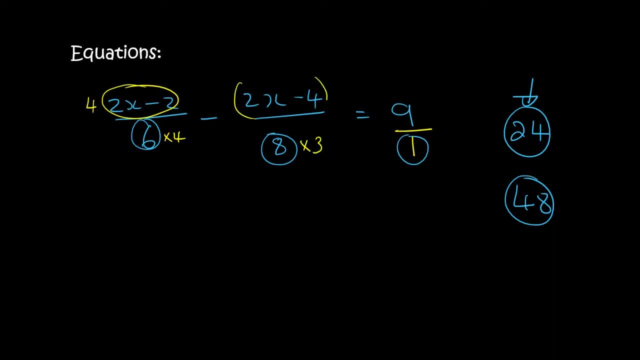 We're going to have to multiply by 3 here to get to 24.. So this one's also going to need a 3.. And then this one is going to need to be multiplied by 24.. Wow, it's going to become a big number. 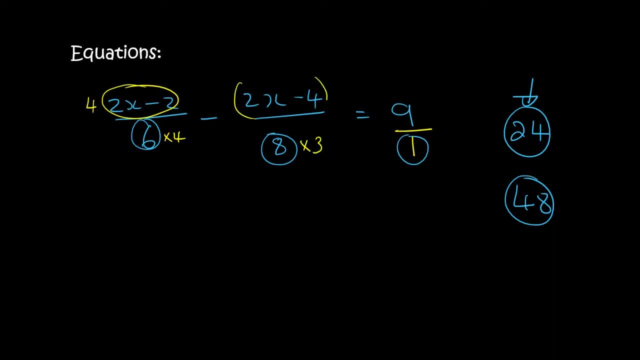 We're going to have to multiply by 3 here to get to 24.. So this one's also going to need a 3.. And then this one is going to need to be multiplied by 24.. Wow, it's going to become a big number. 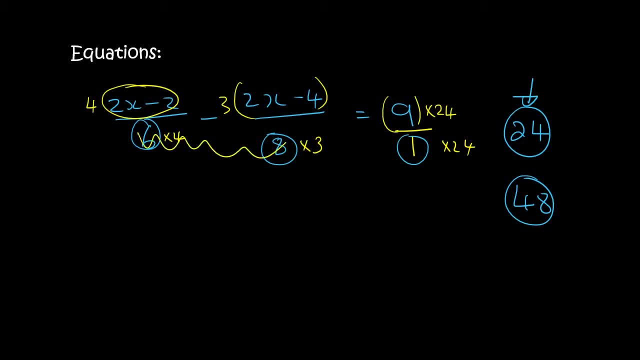 See, because we're multiplying top and bottom, but we don't care about the bottom anymore because we have an equation, We only care about the top. So We now have 4, bracket 2x. I cannot stress the importance of a bracket. 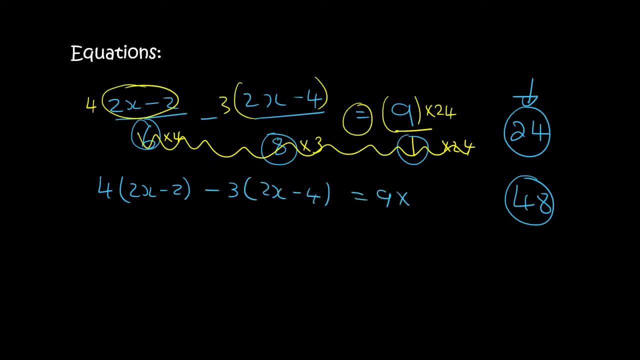 It can actually make your entire question incorrect if you don't use it. Okay, so now we multiply the 4 in, So that becomes 8x minus 8 minus 6x, and then this minus and that minus becomes plus 12.. 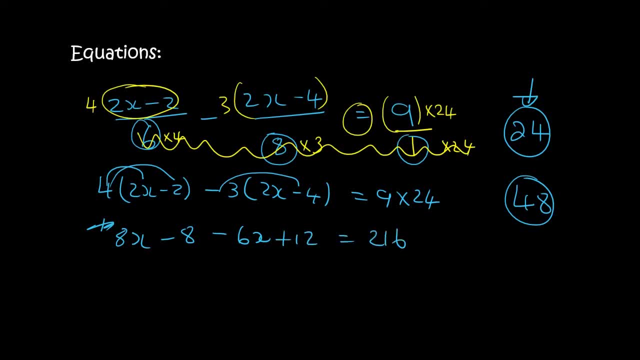 9 times 24, 216.. Okay, so now we can take all the x's: The x's to the one side and all the numbers to the other side. So I'm going to take these two numbers over here. I'm going to take them over to the right-hand side. 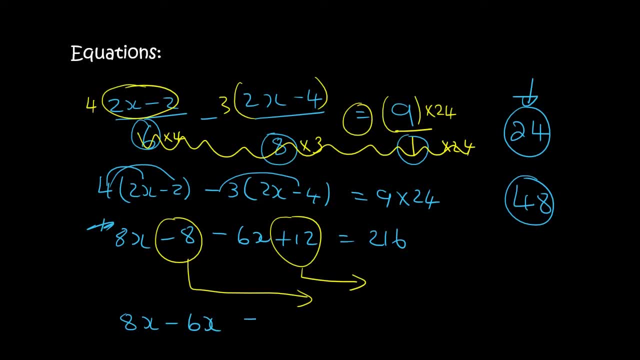 And so on the left we will still have: 8x minus 6x equals 216.. Then when this minus 8 goes over, it becomes plus 8. And this plus 12 will become minus 12.. So 8x minus 6x is 2x. 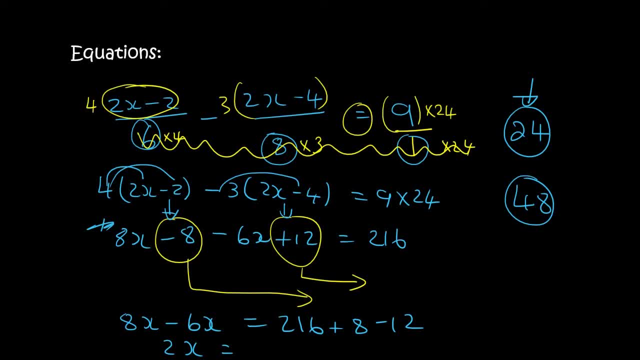 Then on the right-hand side, if we add all of that together, you'll get 212. So at the moment we've got 2x equals to 212.. To get x by itself, you divide both sides by 2 so that this can cancel out. 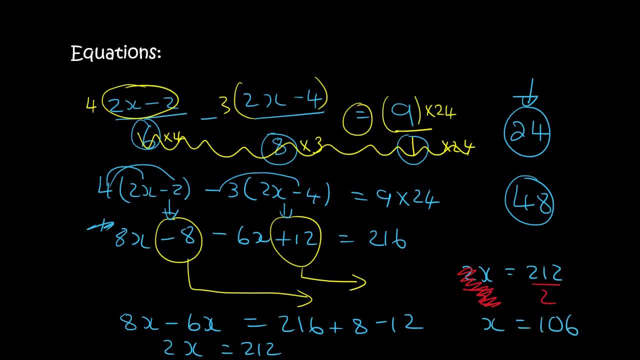 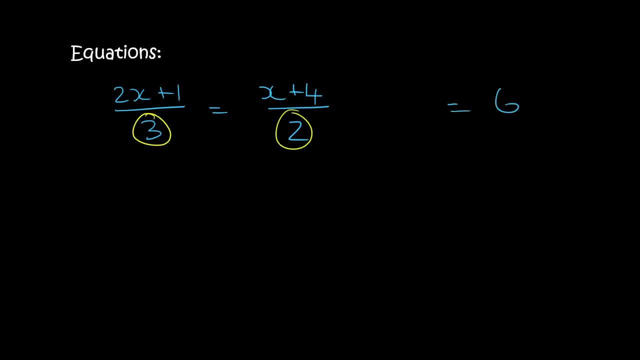 And so x will end up equaling 106.. So here's another one. So here we have a fraction. So you look at the 3 and the 2, and the common number that could link those is 6.. But if you wanted to choose 12, that's also fine. 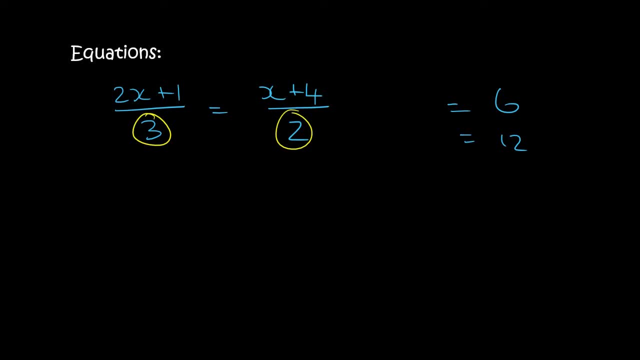 No one's judging you, You do you. So to get From 3 to 6, you would multiply by 2.. And so we're also going to multiply this one by 2.. And you'd multiply this one by 3.. 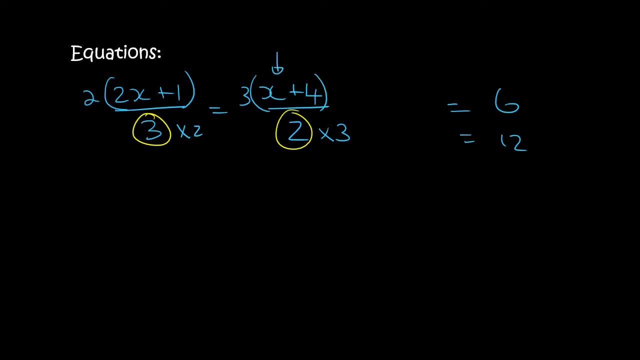 And so you'd also multiply this one by 3.. Important guys, Use the brackets. Trust me, Then, because these are now both going to be a 6, you can ignore them, And so what we have is 2 to the 2x plus 1 equals to 3 to the x plus 4.. 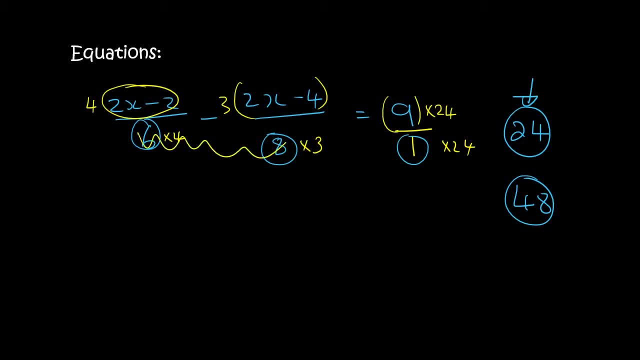 See, because we're multiplying top and bottom, but we don't care about the bottom anymore because we have an equation, We only care about the top. So We now have 4, bracket 2x. I cannot stress the importance of a bracket. 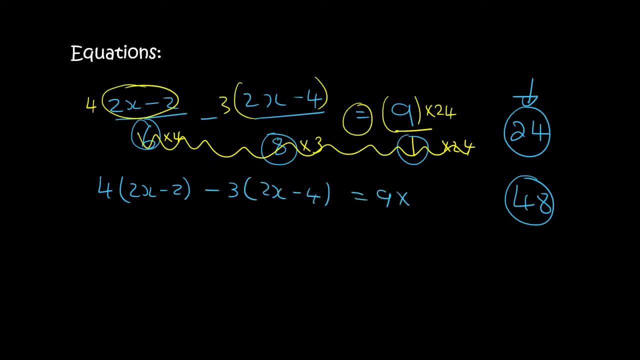 It can actually make your entire question incorrect if you don't use it. Okay, so now we multiply the 4 in, So that becomes 8x minus 8 minus 6x, and then this minus and that minus becomes plus 12.. 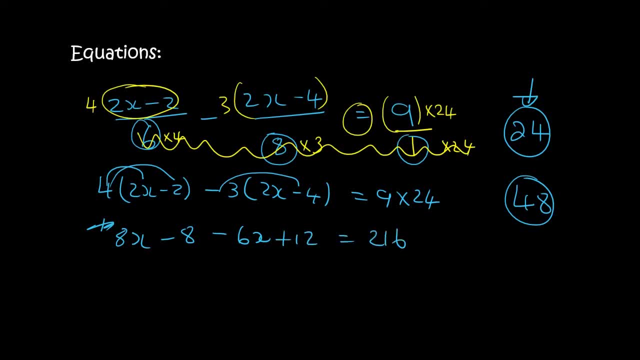 9 times 24, 216.. Okay, so now we can take all the x's: The x's to the one side and all the numbers to the other side. So I'm going to take these two numbers over here. I'm going to take them over to the right-hand side. 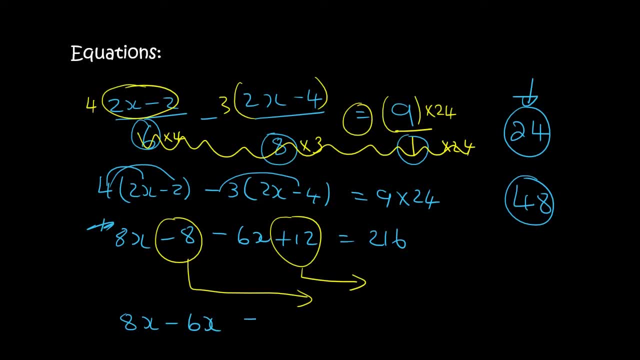 And so on the left we will still have: 8x minus 6x equals 216.. Then when this minus 8 goes over, it becomes plus 8. And this plus 12 will become minus 12.. So 8x minus 6x is 2x. 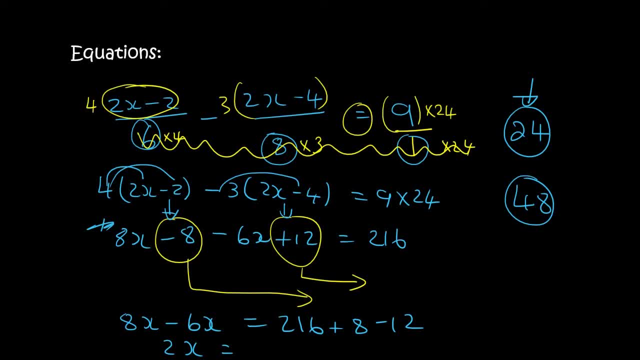 Then on the right-hand side, if we add all of that together, you'll get 212. So at the moment we've got 2x equals to 212.. To get x by itself, you divide both sides by 2 so that this can cancel out. 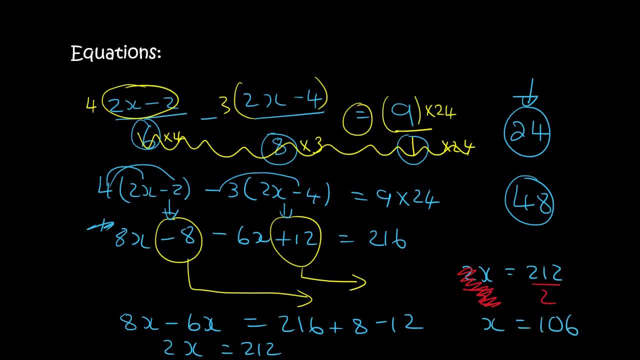 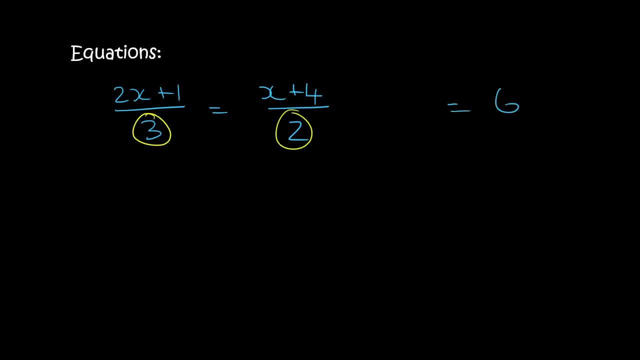 And so x will end up equaling 106.. So here's another one. So here we have a fraction. So you look at the 3 and the 2, and the common number that could link those is 6.. But if you wanted to choose 12, that's also fine. 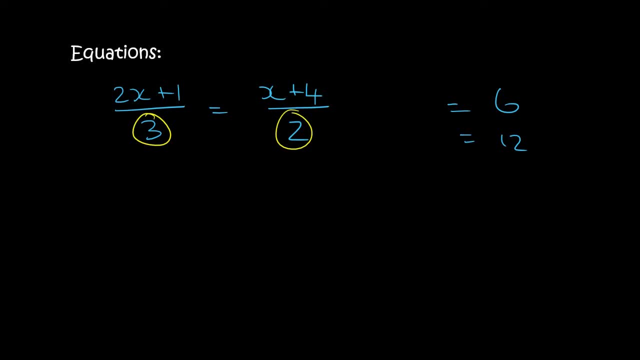 No one's judging you, You do you. So to get From 3 to 6, you would multiply by 2.. And so we're also going to multiply this one by 2.. And you'd multiply this one by 3.. 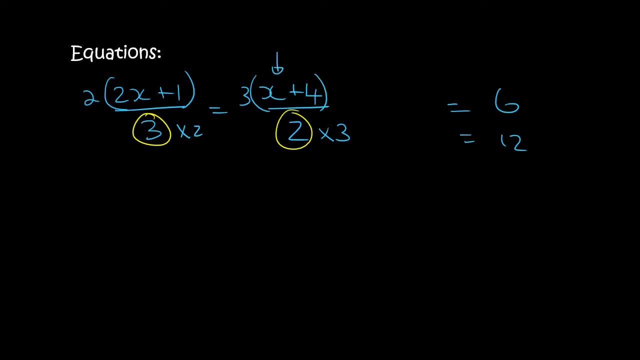 And so you'd also multiply this one by 3.. Important guys, Use the brackets. Trust me, Then, because these are now both going to be a 6, you can ignore them, And so what we have is 2 to the 2x plus 1 equals to 3 to the x plus 4.. 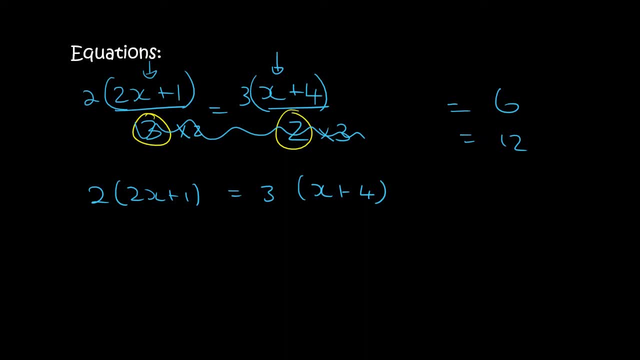 And then you just multiply in. So I'm not going to go any further with this. What I'm going to now practice for the rest Of this lesson is just helping you guys to do this part, Because by now you know how to do this part over here. 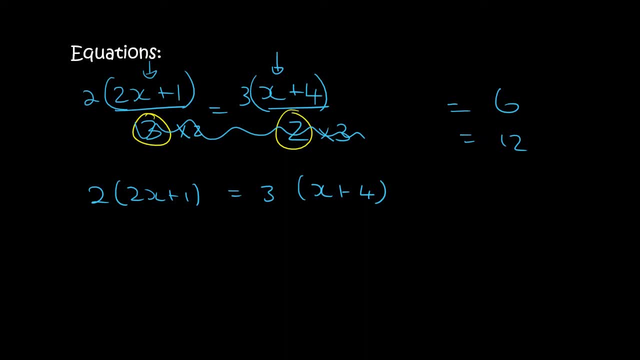 And then you just multiply in. So I'm not going to go any further with this. What I'm going to now practice for the rest Of this lesson is just helping you guys to do this part, Because by now you know how to do this part over here. 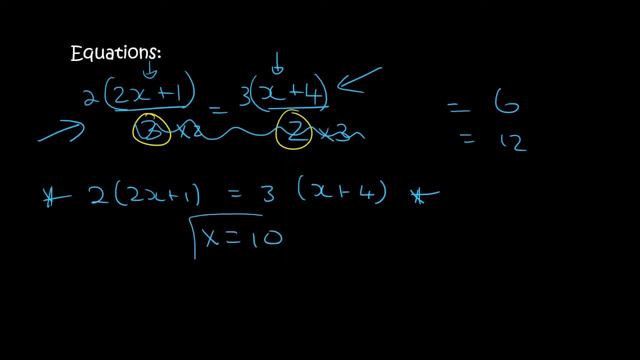 But if you do want to carry on with this one, your answer that you should get is 10.. So if you get to that, good for you. Here's another one. So why not pause the video and see how far you can get with this one? 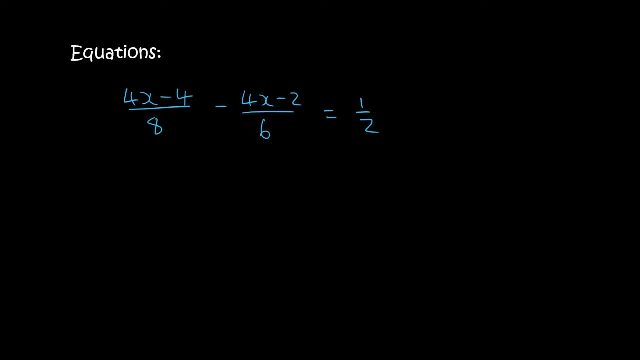 So if you look at the numbers 8,, 6 and 2, your common denominator is going to be: You could use 24.. And so that means This one needs to be multiplied by 3.. So you just put a little 3 there. 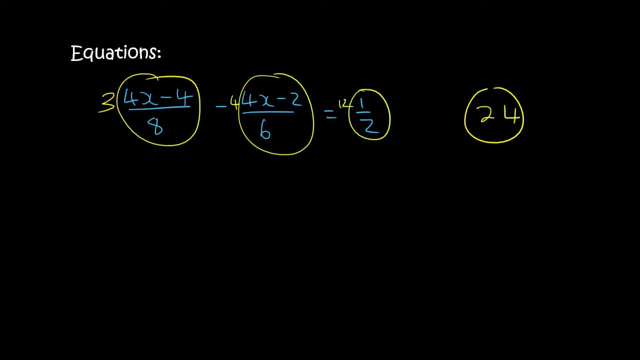 This one needs to be multiplied by 4. And this one needs to be multiplied by 12.. So all that that means is you're now going to end up with 3 bracket 4x minus 4 minus 4. bracket 4x minus 2 equals 12 bracket 1.. 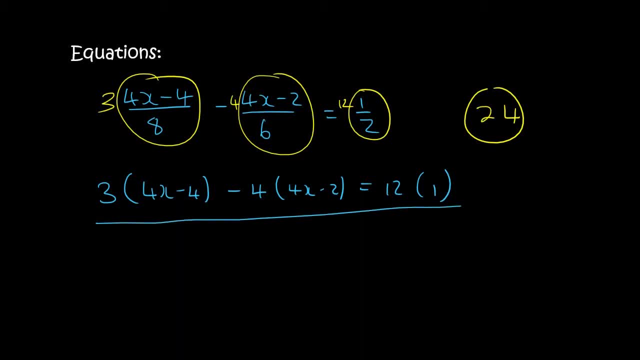 That is it, guys. It's that simple. At this point, you guys know what to do, So I'm not going to go any further with that. What's important now is how to do this top part. Okay, So here's another one. There's fractions. 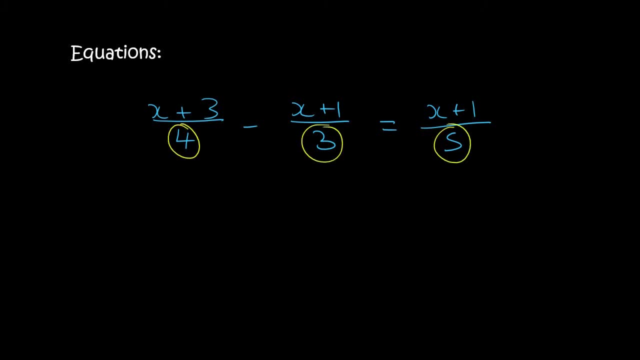 So the lowest number that could link 4, 3 and 15 would have to be- I'm just going to go with- 60. Maybe there's a lower number, I don't really know. Well, I'm not going to waste time trying to find that. 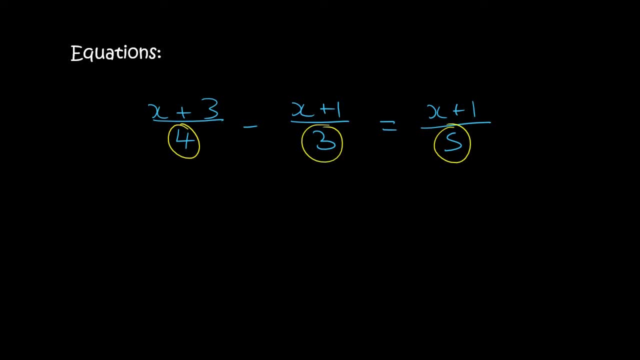 I'm just going to go with 60. So I know that if I times 4 by 15, I would get 60. So I could put a 15 here, then a bracket- Very important- This one- I'd need to multiply by 20.. 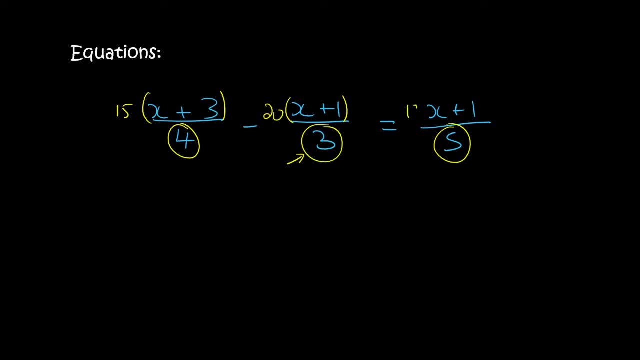 So I put a bracket and this one I'd need to multiply by 12, and then I put a bracket, So at that point you would have 15x plus 3 minus 20. bracket x plus 1 equals to 12 bracket x plus 1.. 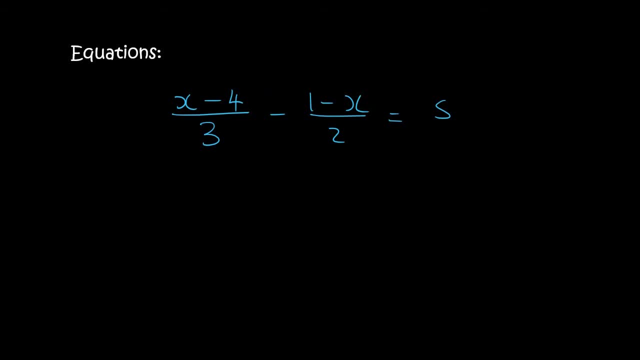 And then at this point it should be fairly straightforward. Okay, This will be the last one, So always remember that this number also needs to be included. So here we've got 3 and 2, so the common denominator is going to be 6.. 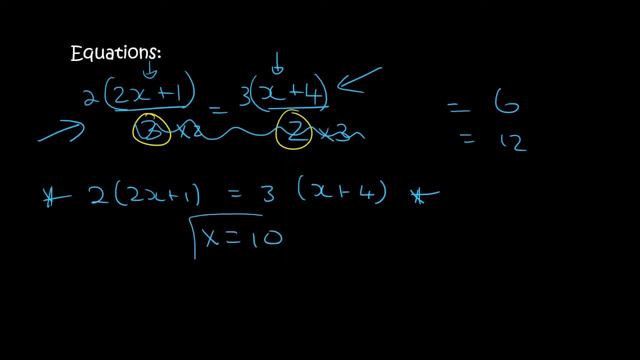 But if you do want to carry on with this one, your answer that you should get is 10.. So if you get to that, good for you. Here's another one. So why not pause the video and see how far you can get with this one? 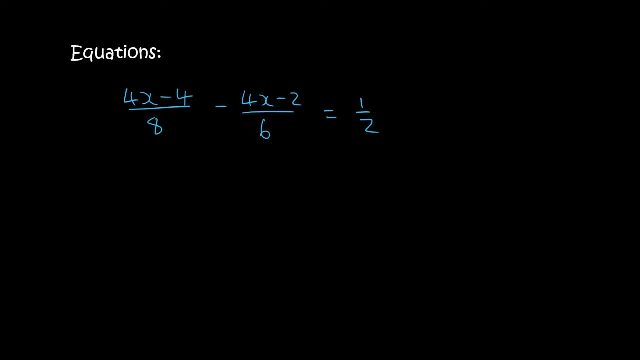 So if you look at the numbers 8,, 6 and 2, your common denominator is going to be: You could use 24.. And so that means This one needs to be multiplied by 3.. So you just put a little 3 there. 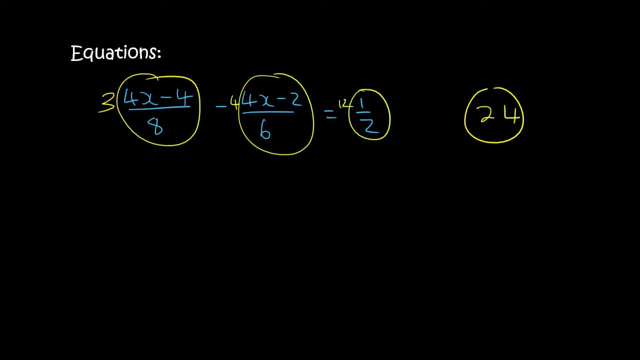 This one needs to be multiplied by 4. And this one needs to be multiplied by 12.. So all that that means is you're now going to end up with 3 bracket 4x minus 4 minus 4. bracket 4x minus 2 equals 12 bracket 1.. 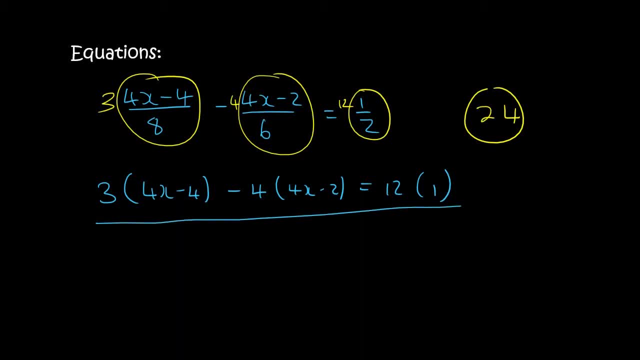 That is it, guys. It's that simple. At this point, you guys know what to do, So I'm not going to go any further with that. What's important now is how to do this top part. Okay, So here's another one. There's fractions. 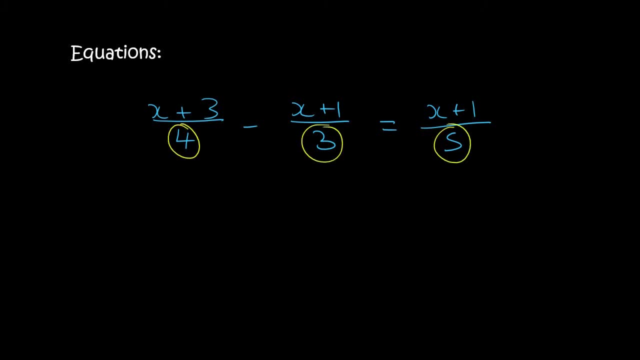 So the lowest number that could link 4, 3 and 15 would have to be- I'm just going to go with- 60. Maybe there's a lower number, I don't really know. Well, I'm not going to waste time trying to find that. 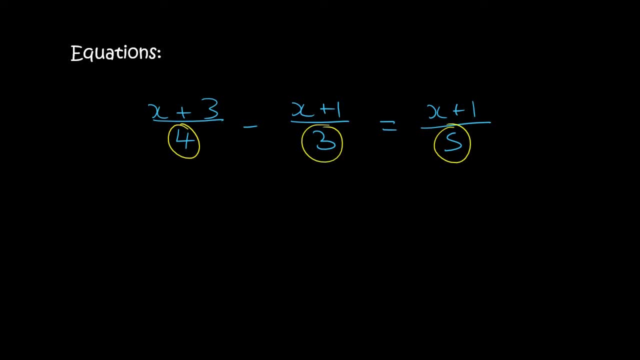 I'm just going to go with 60. So I know that if I times 4 by 15, I would get 60. So I could put a 15 here, then a bracket- Very important- This one- I'd need to multiply by 20.. 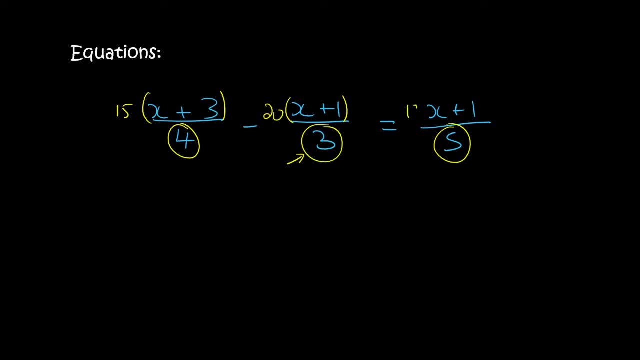 So I put a bracket and this one I'd need to multiply by 12, and then I put a bracket, So at that point you would have 15x plus 3 minus 20. bracket x plus 1 equals to 12 bracket x plus 1.. 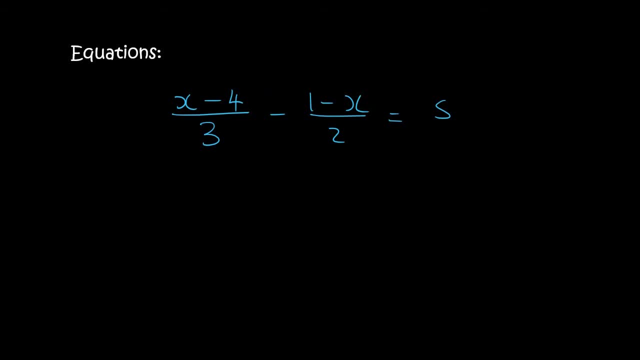 And then at this point it should be fairly straightforward. Okay, This will be the last one, So always remember that this number also needs to be included. So here we've got 3 and 2, so the common denominator is going to be 6.. 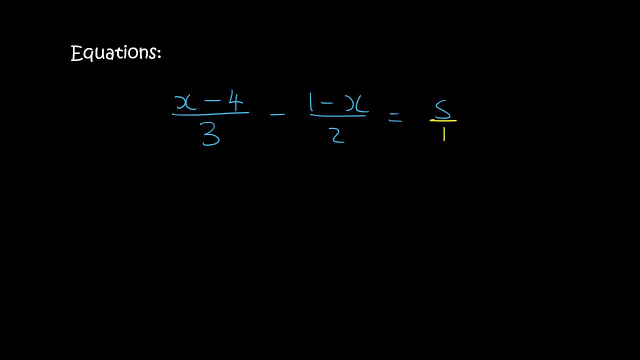 So. but if you chose 12,, it's okay. If you chose 24,, if you chose 18, it doesn't matter, because at the end the answer will simplify. So where your friend might get 2x equals to 4 at the end.